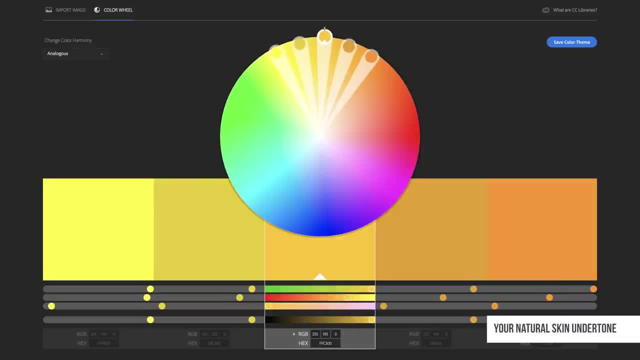 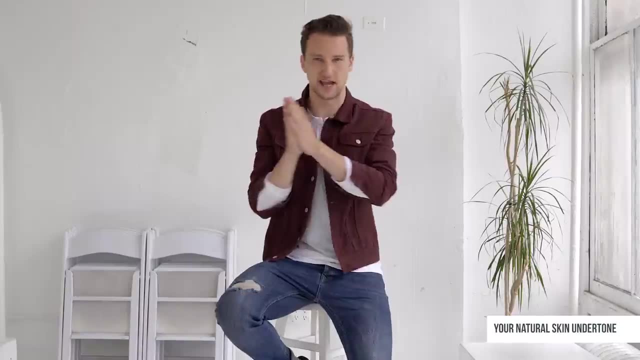 If you're on the warmer side of your skin tone, then you're going to want to stick to the warmer half of the circle. I want to share that with you guys because I think it's important to know. I myself I put myself somewhere in the middle of that scale between yellow and blue a little bit. 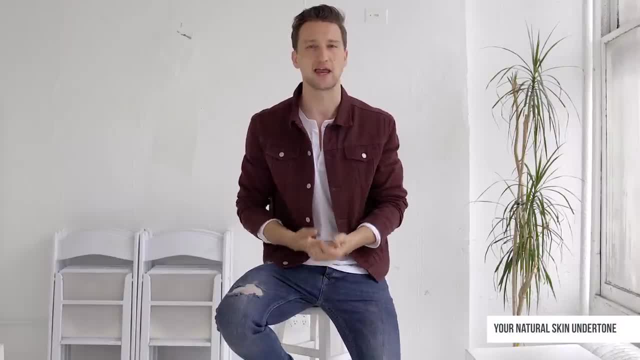 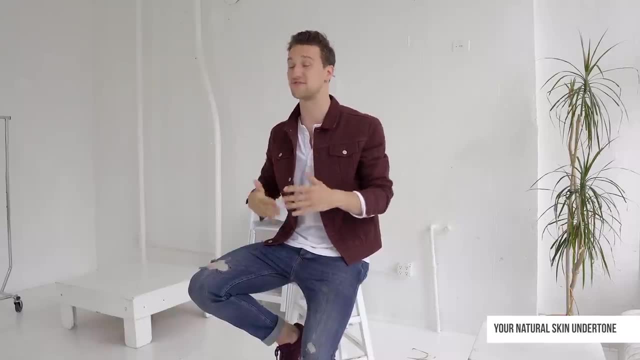 more on the colder side, But at the same time I think any guy can wear any color in the right: hue, saturation and lightness. Now I just threw three terms at you that define color. Any color is made up of the hue, the general color that it is, the saturation of it. so 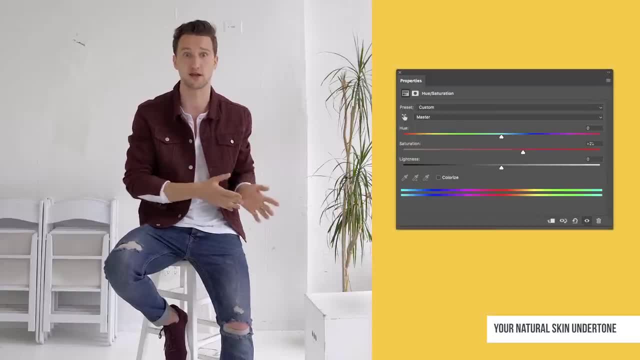 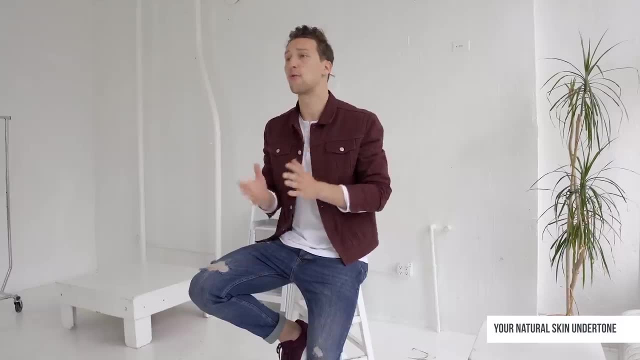 how bold it is, how rich it is, or how dull it can be, how saturated it is. I feel like you guys probably know what that means and how light or dark it is. It's the luminance of a color. So, while I want you to keep this basic approach of your skin tone in mind, we're going to 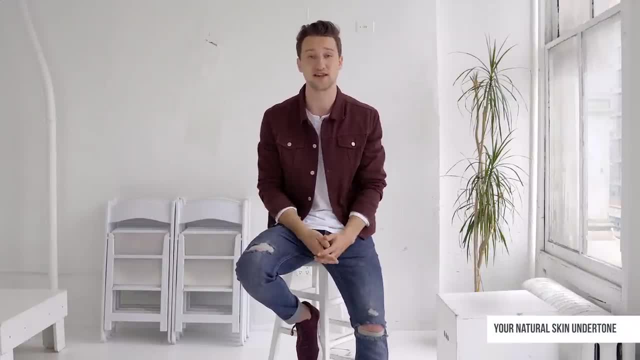 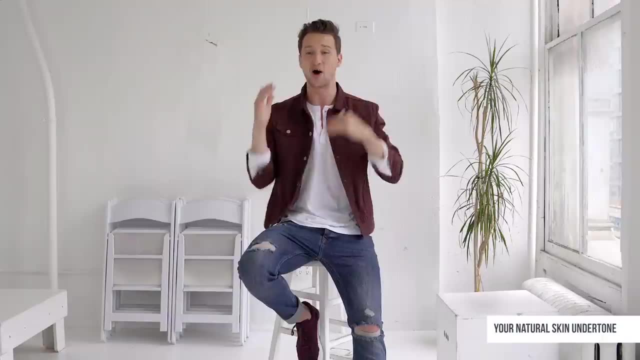 be talking about a bunch of colors today and just a general approach on how to integrate them into your outfit. My channel is much more focused on fashion, and every season you have different colors that are trending, so I want to inform you guys on how to think about those colors, how. 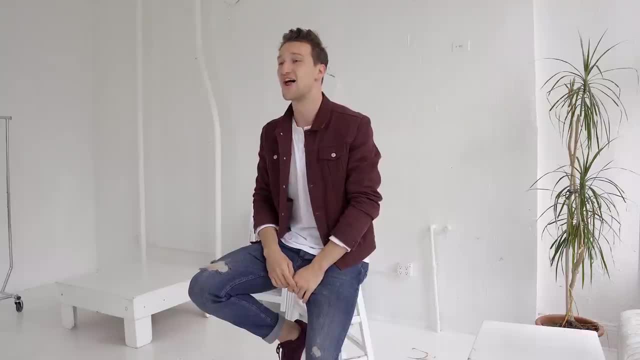 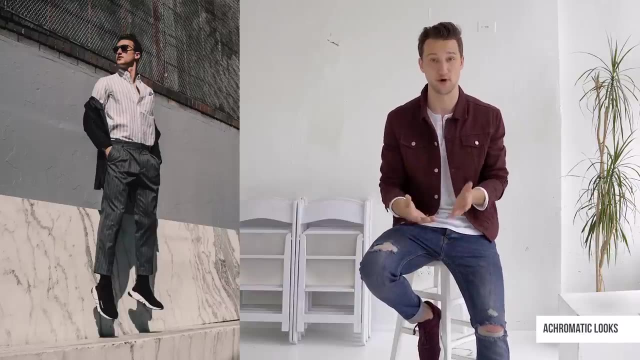 you can integrate those into your outfits and into your wardrobe. So let's look at it specifically, starting with this look first. Let's take a look at this first outfit and the underlying approach to it, which is a lack of color. It's an achromatic look. 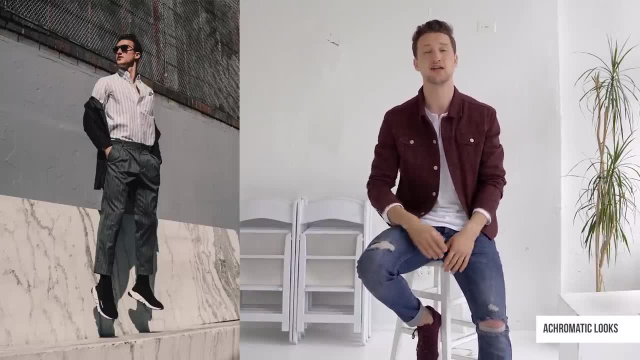 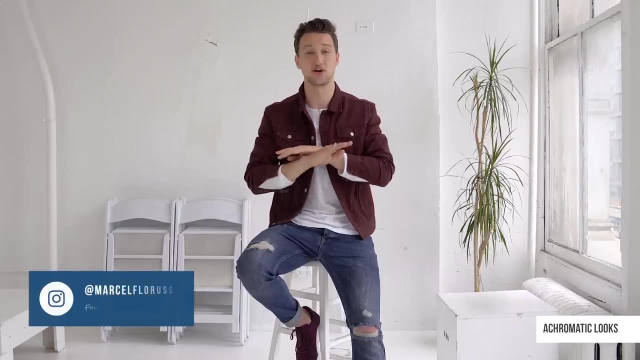 It's one of the easiest things to pull off, because you don't have to worry about matching colors. White and gray and black aren't colors, they're contrasts. To be precise, white actually is all colors combined and black is literally no color. 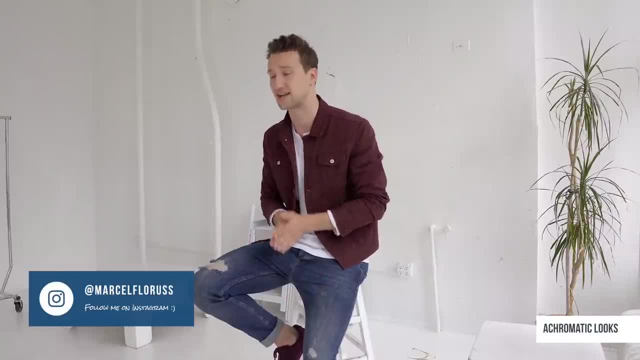 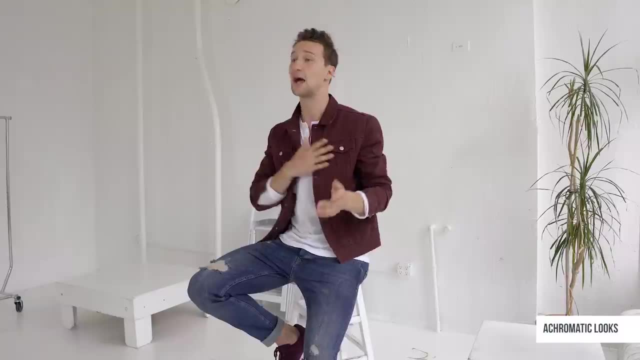 For the sake of this video, I'm going to refer to them as colors, but know that they're technically called contrasts. What's important here is, like I said, you don't have to worry about matching it so much, but it is about contrast. 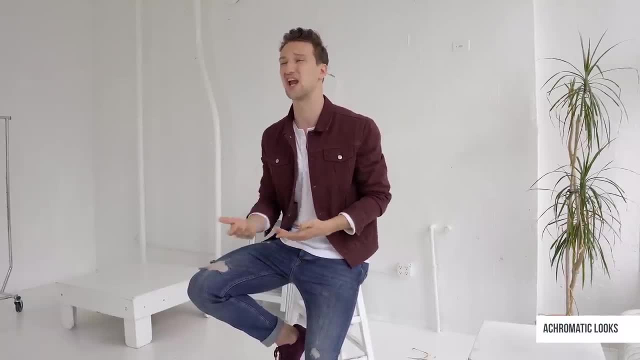 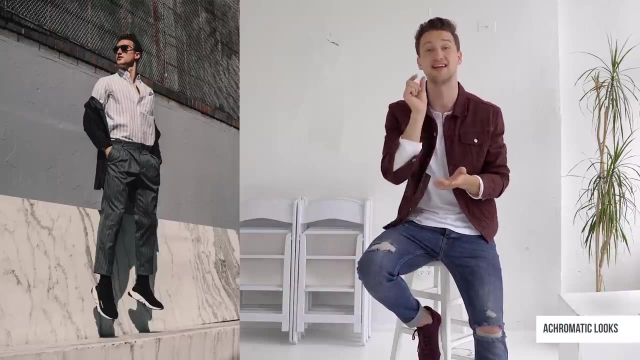 I personally, when I wear an achromatic look, don't like to go for a very high contrast ensemble. Starting off the look here that we have as an example, we have gray pants with white stripes, then we have a white shirt with light gray stripes and a black coat and black sneakers. 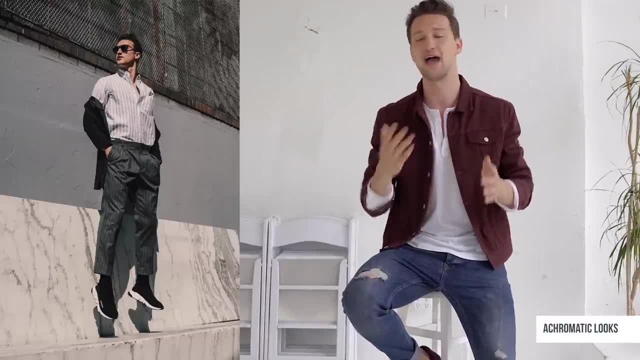 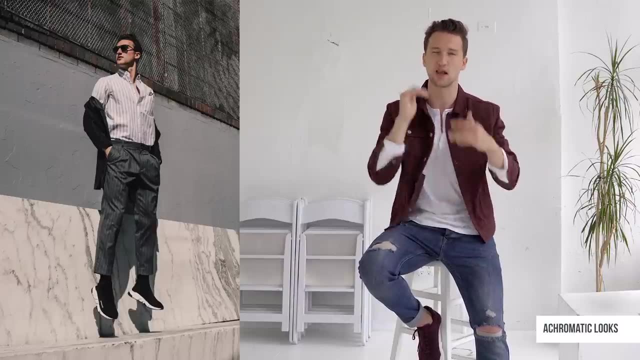 tying it all together. So I'm kind of leveling the contrast out. I rarely I will, but I rarely will wear black sneakers and white jeans and like a black top. again, It's a lot of contrast for me, but I think this goes back to personal preference. 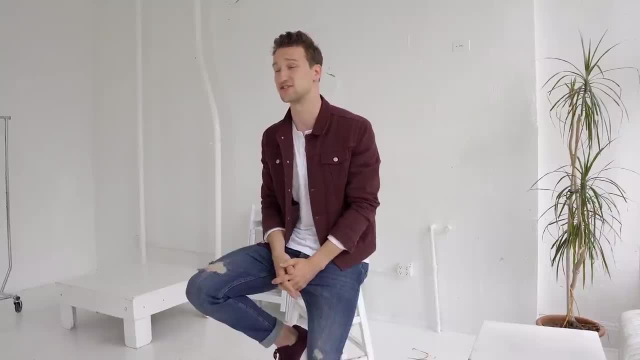 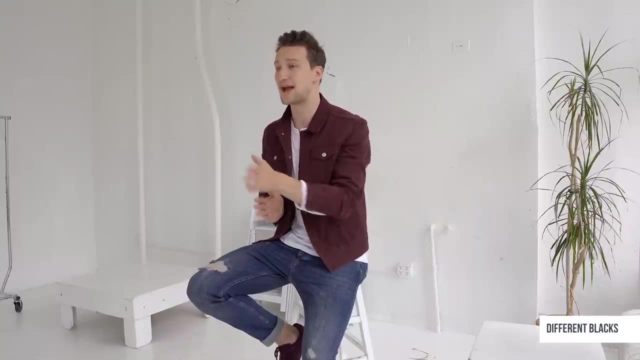 But just know that with an achromatic look, that's one of the main considerations If you want to just wear black. really important note, And this goes for all colors: They don't always look the same. Black isn't black isn't black. 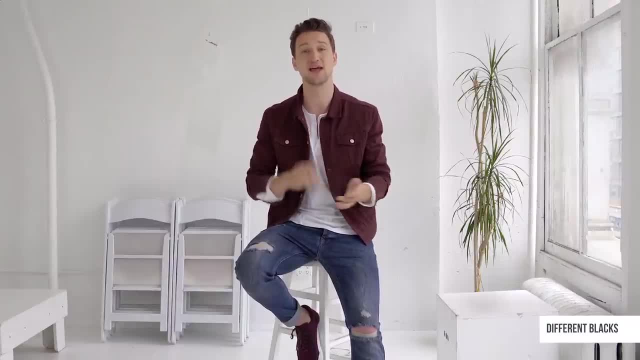 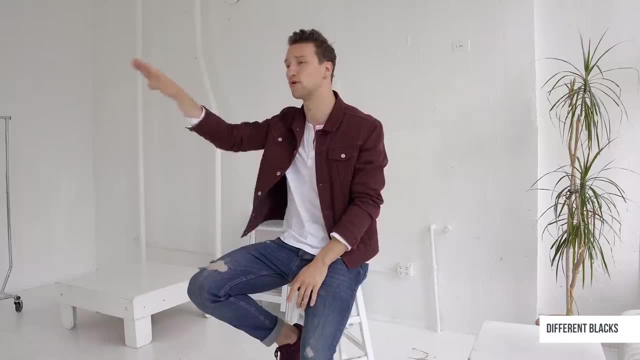 It depends on the fabrication, It depends on the light source hitting the garment and it depends on the quality of the dye of the garment. This is especially important when you're trying to shop for a suit and you think, oh cool, this suit jacket is on sale and these suit pants are on sale. 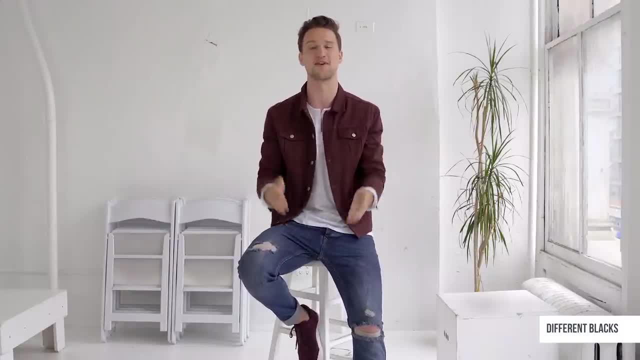 They're both black. It'll be fine. It won't be, Trust me, especially when you step in front of a flashlight, one of the least forgiving light sources, because it really blows out the color, or, in this case, the black. 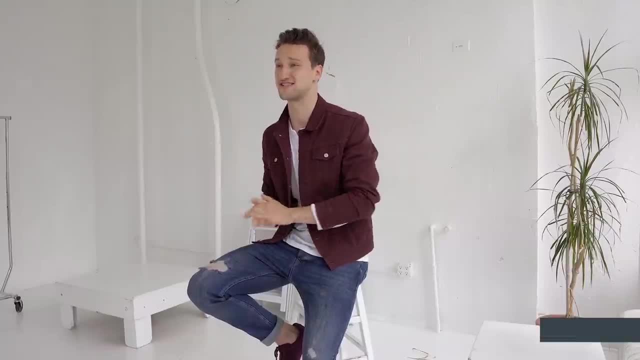 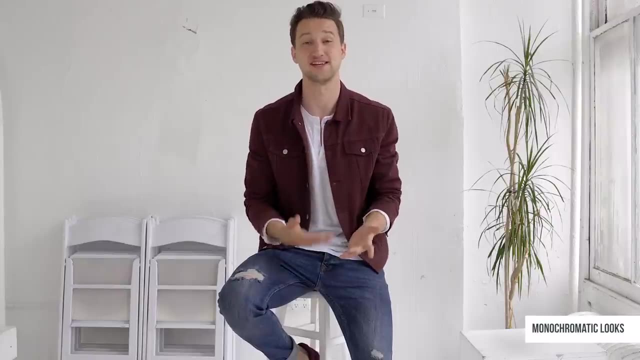 Either it's matching perfectly or there has to be enough contrast in your look to make that work. The second way to approach making an outfit would be to take one color, and this happens to be a spring trend: monochromatic dressing. It's a very simple approach. 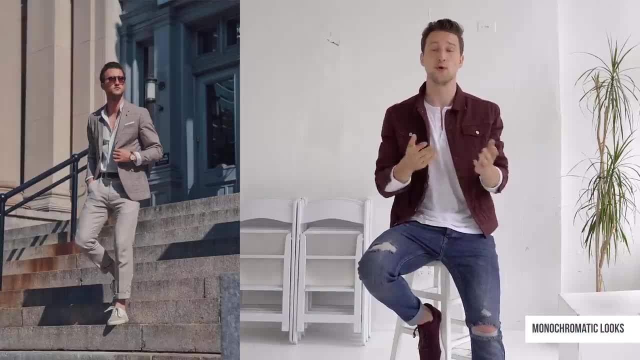 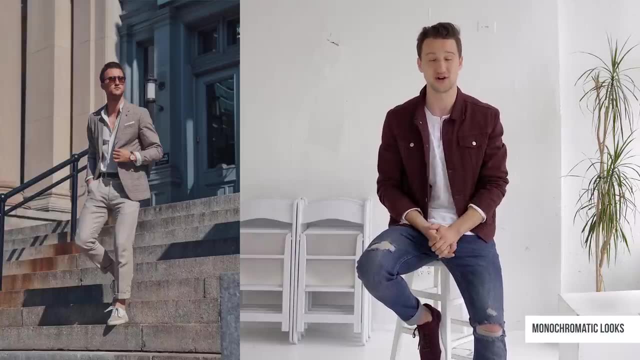 Take this look, for example, one of the outfits from my recent Zahara lookbook, where we have beige pants, we have a beige, a little darker beige- blazer and a white and beige striped shirt with white and beige sneakers. So, as you can see, the main color would be beige. 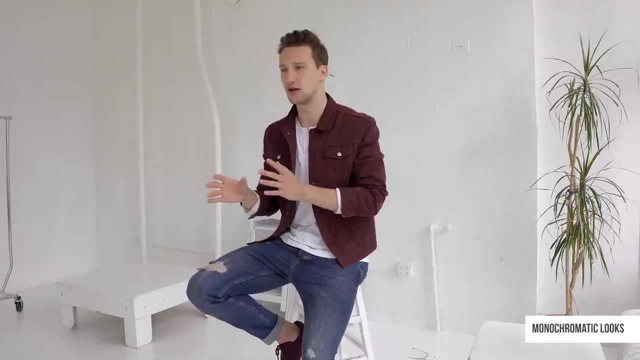 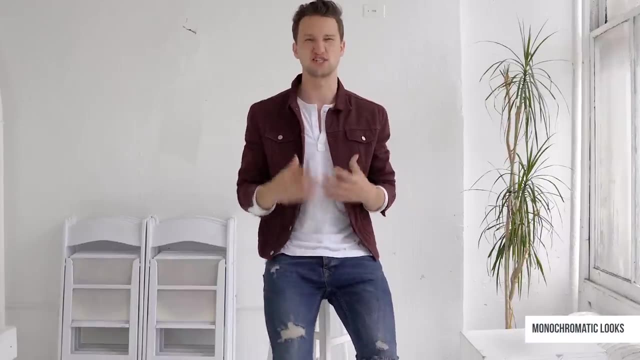 But I'm adding some white in there which is close enough to it, And with monochromatic dressing you can add whites and grays and blacks into it fairly easily and still have it just be about that one color. But here, similarly to the achromatic looks, you want to make sure that there's enough. 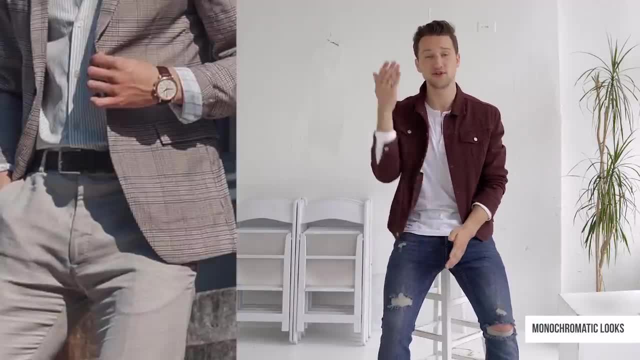 contrast between the pieces. Take the pants and the blazer, for example. If you just take the base color of the blazer they're actually really similar, But the pattern of the blazer, which is actually darker, makes the overall blazer a little. 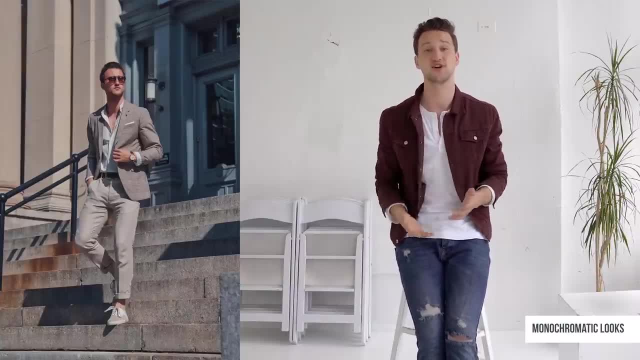 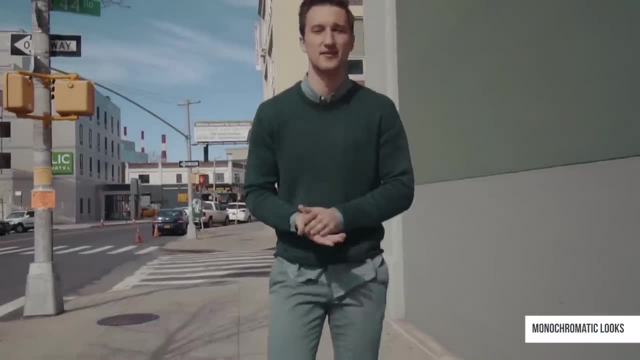 bit darker And thus there's more contrast between the pants and the blazer, And that's why it works. Another example would be the look that I have in my spring trend video for monochromatic dressing: This look from Club Monaco. 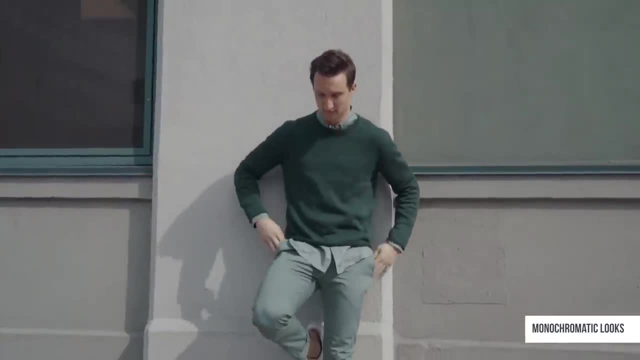 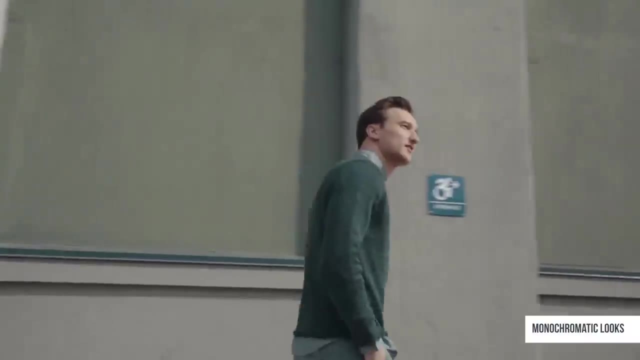 The main color here is green And you can see that the chinos and the shirt are actually almost identical. But then the darker, more rich, deeper green of the sweater really breaks them up, adds a little bit more contrast and really makes for a true monochromatic look. 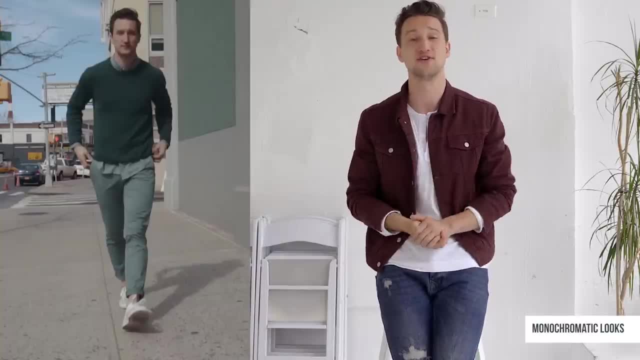 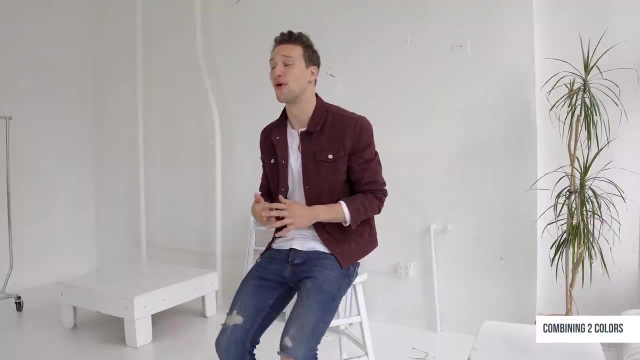 Here we don't even have any white in there, It's literally just green on green on green, but different shades of it to create a trendy seasonal look That I personally love, Systematically adding more colors. here let's talk about a two-color approach. 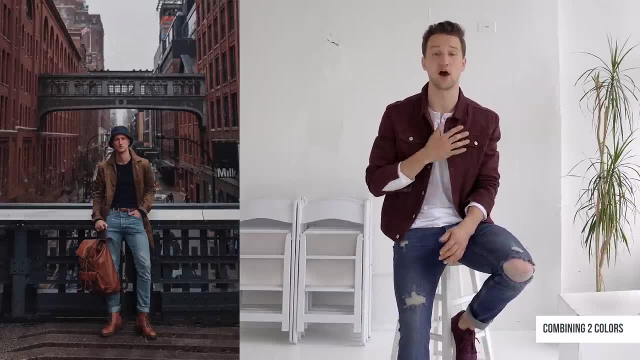 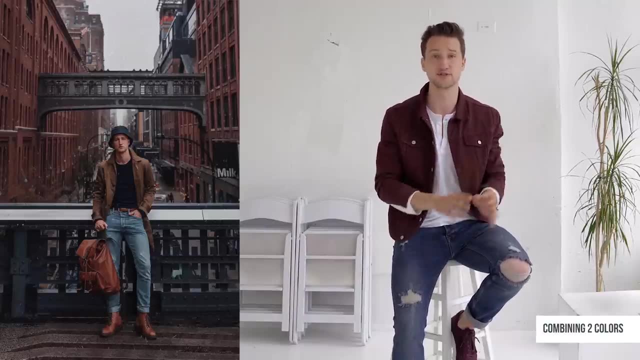 This outfit. here is two main colors, blue and brown, which I think are very complementary, And I like combining those a lot. Most of my wardrobe is somewhere in the earth tones and in the navies and blue tones, So here we have a light wash jean together with a dark blue knit sweater on the blue. 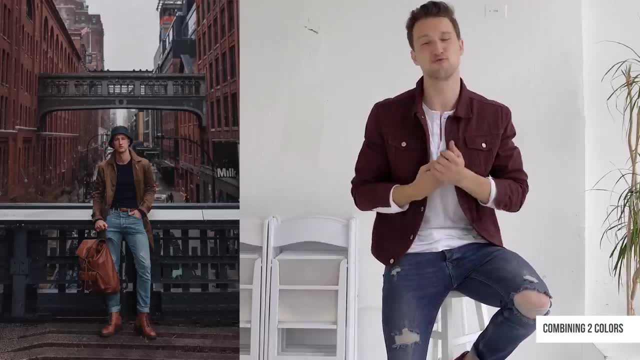 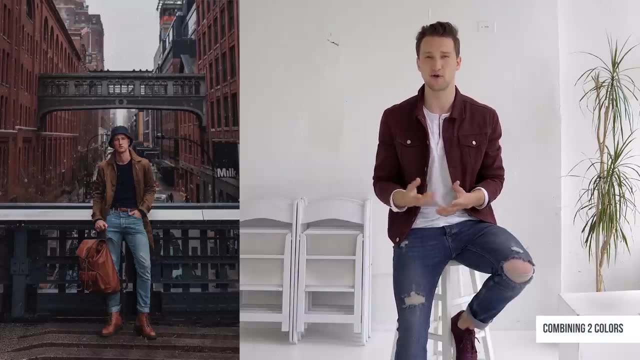 side of things. And then, on the brown side of things, we have three rich cognac colors that are matching in the backpack, The belt And the boots, And then we have a more greenish brown in the raincoat, which still works because it's. 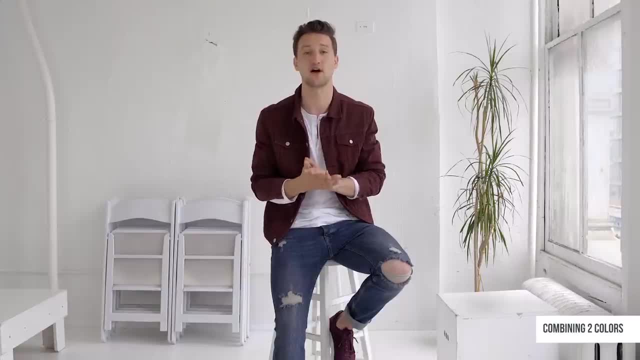 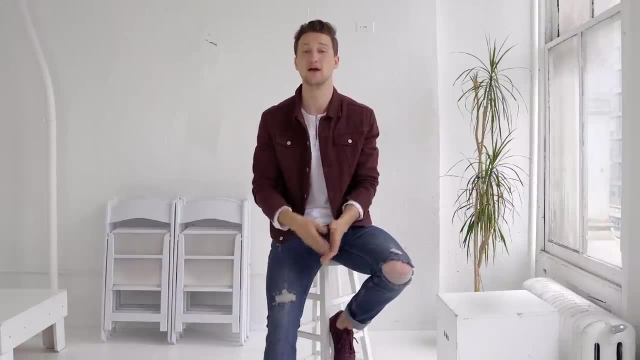 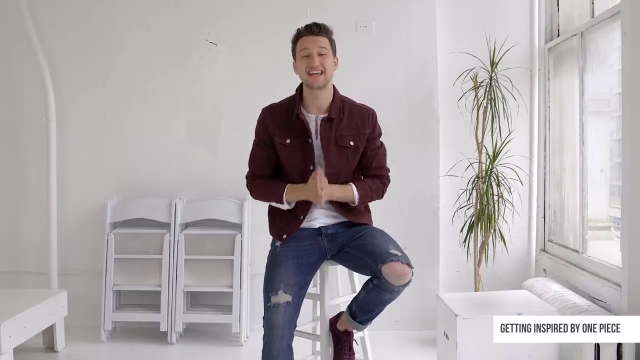 in the earth tone range and they're different enough. Once again, there's enough contrast between the browns and between the blues in their separate categories And then combining them just works, because brown and blue are very, just, very complementary colors. And this is step number four: getting inspired by one piece and its color scheme. 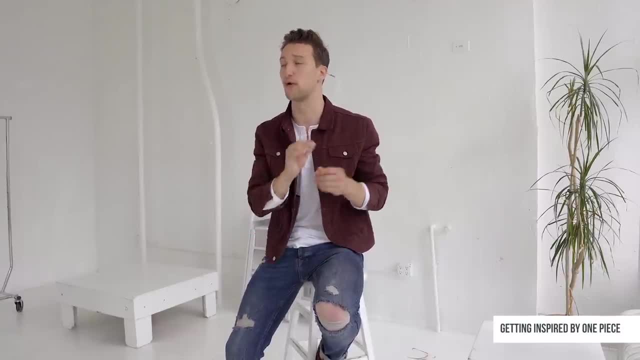 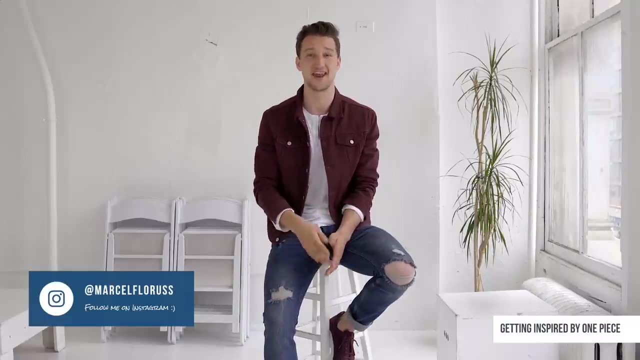 So really, what you're doing is just trusting the designer. You put one piece together to know what they were doing in terms of color, because obviously they're in design and they've studied it and they know what they're doing most of the time. 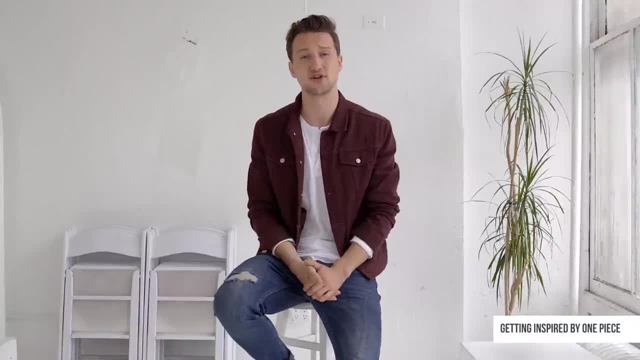 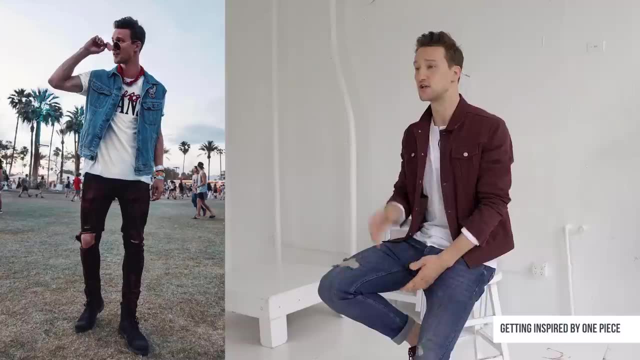 So what you do is you take their design apart. Take this look from Coachella last year, for example, I wore a basic white t-shirt from Guess that had a black and red font across the chest, So the white was already pretty predominant. 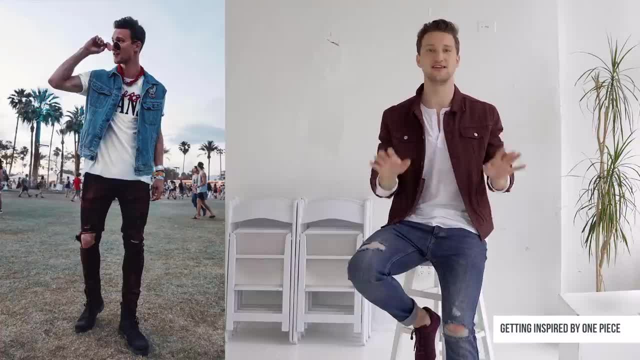 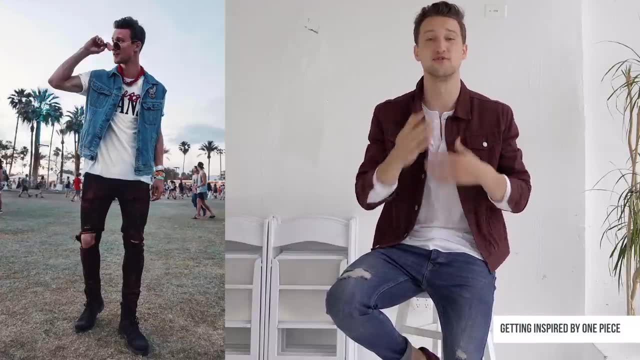 So I wanted to pick up the black and red and it was Coachella. So I'm wearing crazy tie dye black and red jeans that are ripped, but I'm wearing black boots, I'm wearing a red bandana and even the patch on the denim vest is red to really tie that. 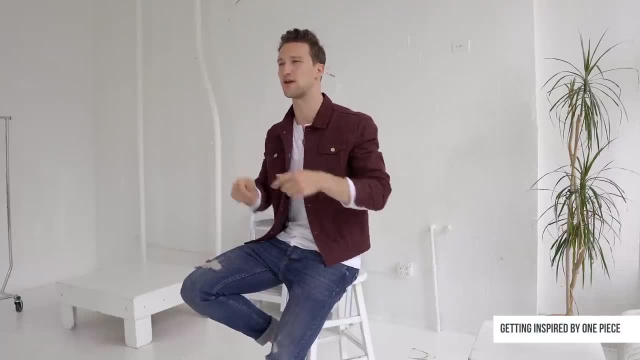 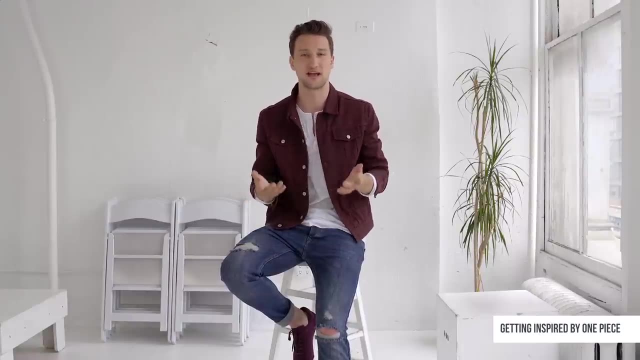 in Denim I would always consider a neutral in fashion. You can kind of throw it in any look and it just works, even though it's technically blue. So that's why it worked for me here. I just threw that in as a little bit of a little bit of an extra, but even that piece. 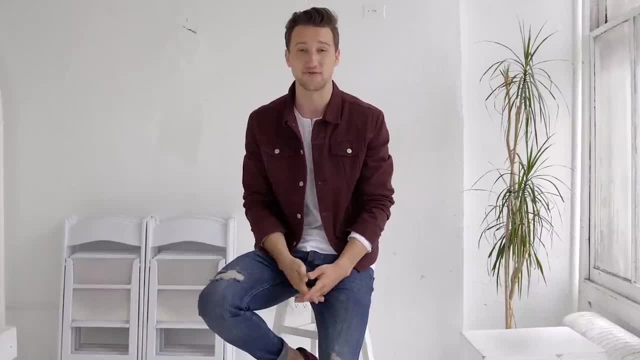 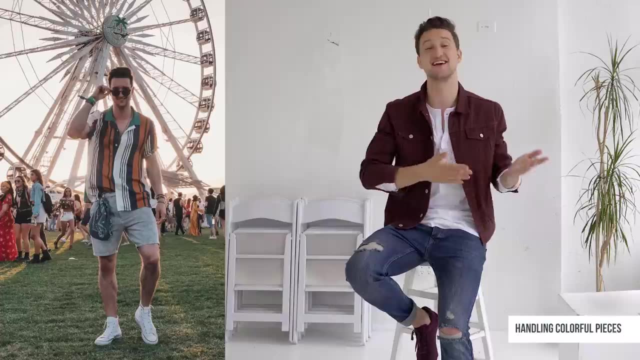 is integrated into that color scheme. So that's a way to think about making an outfit and really just trusting the designer and following their lead. Step number five Now, if a designer really likes colors and he creates something like this, another Coachella look. 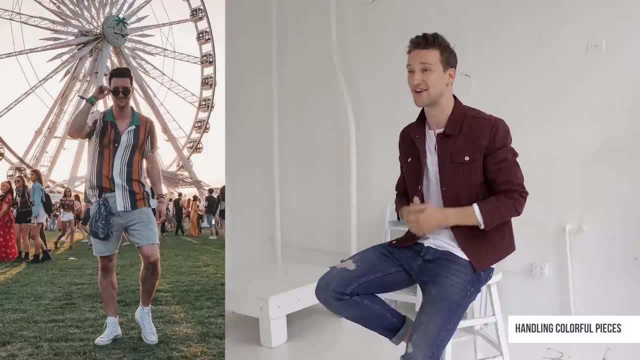 And I did not mean for them to be back to back What happened. This is from this year and I love this top man shirt. It's amazing, but you've got blue in there, yellow, green and even some purple on the. 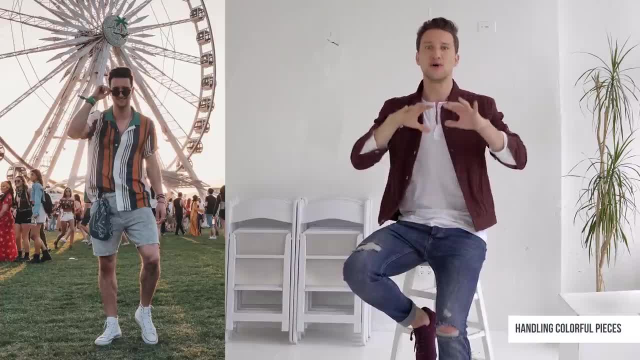 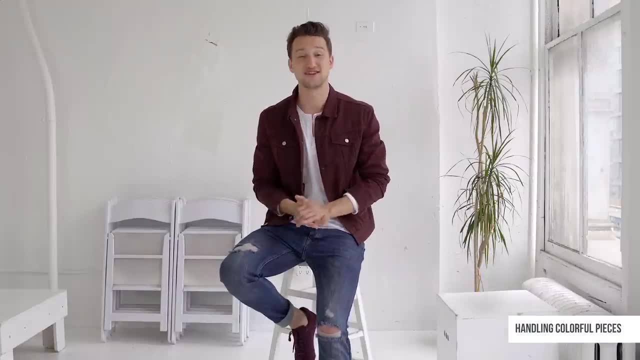 inside of my sleeve. If you look very closely, it's more more on the back, So it's a crazy amount of colors really, especially for somebody like me. I usually go for more muted tones. What do you do? You try to dress it down. 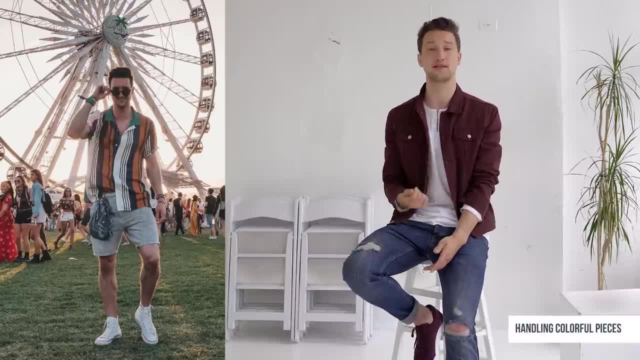 So I'm wearing light gray jean shorts and I'm wearing white sneakers. If you want to pick the color back up, do it in a small way. Maybe wear a bracelet that picks up on the green, or maybe wear shoes that have a blue detail and a similar color. 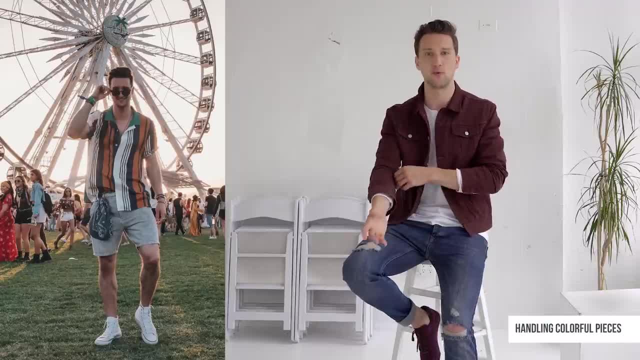 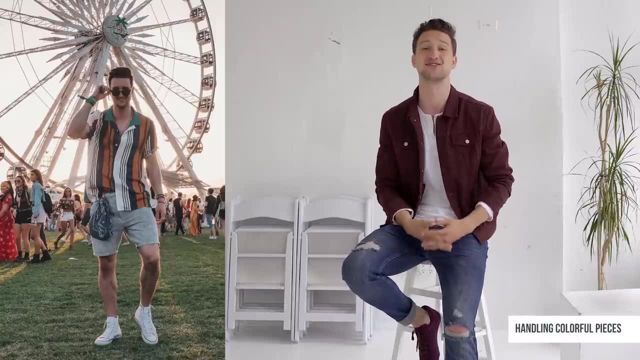 Similar color to what you have in the shirt, but don't be the guy that wears the green matching chinos to the color, because that's just. I mean you can be if that's your thing. Personally, that's not something I go for because I like to tone something. that's that. 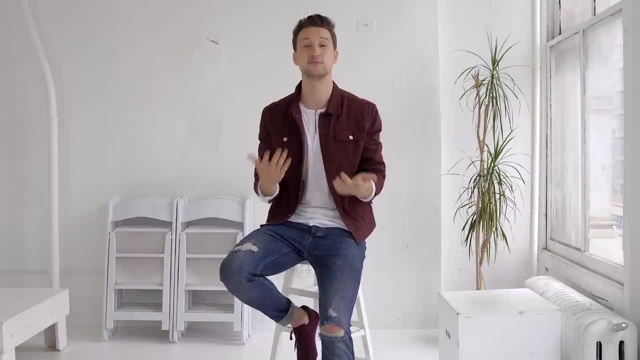 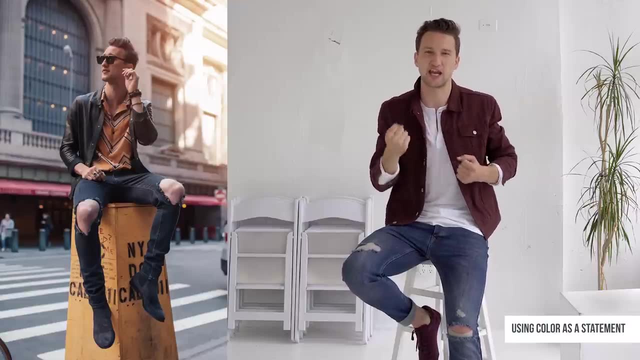 much of a statement, I like to tone down. Number six, And speaking of statements, is using color as a statement. In this look, for example, I have this deep golden, rich like honey, yellow, And that's the main focus. 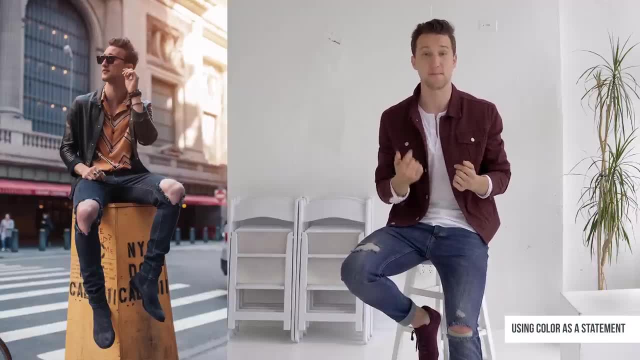 The shirt is from ASOS and the black Chevron stripe. I'm getting inspired What the designer chose, so you can combine several of these approaches too. I chose to just go with an all black outfit around that yellow to really make it pop, to make it stand out by itself and to give it some light to shine. 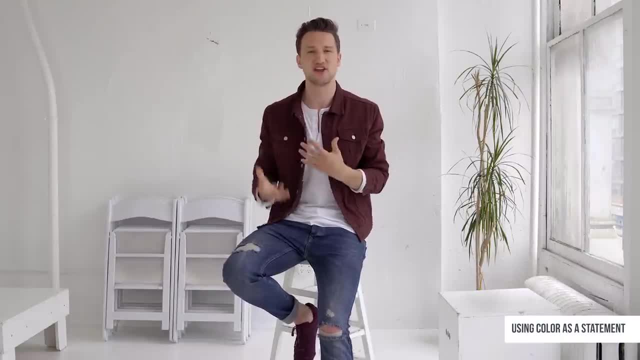 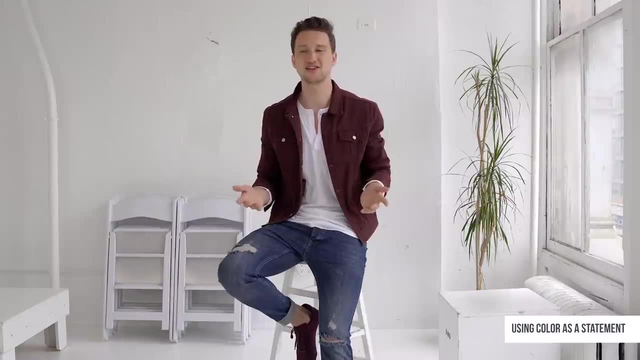 This, for me, is an approach that I have with a lot of, like, very bright colors, very saturated colors, because they are strong already. So, similar to the multicolored shirt, like, just tone it down a little bit. It's actually a really fun way, a really easy way to make a, to make a fun outfit and make 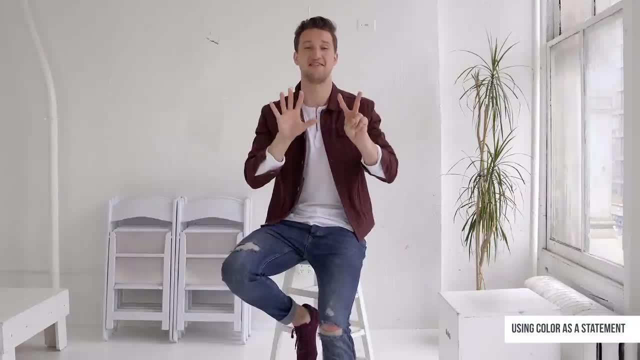 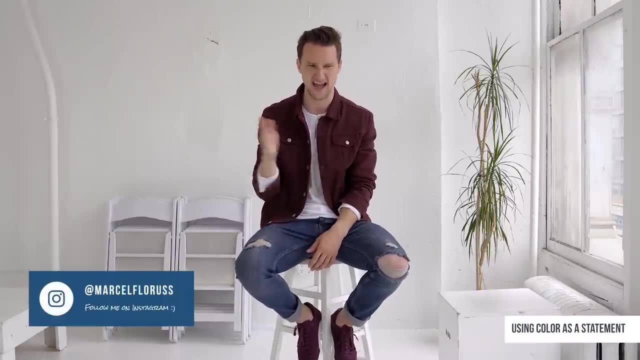 that work, Which already brings us to step number seven, And this one had me baffled. I was going through my Instagram trying to look for outfits literally from the past year for this video, And I looked at this outfit. I'm like no, none of the six principles apply. 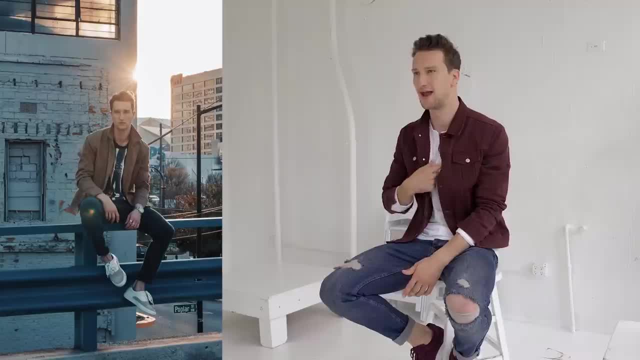 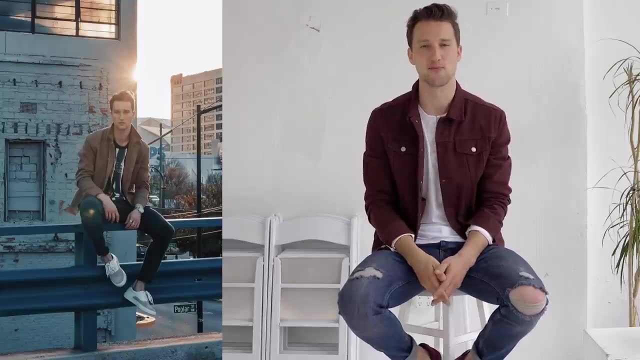 I'm wearing black jeans, I'm wearing a black and green and Bordeaux t-shirt and I'm wearing white and gray sneakers. Why the heck did I decide to wear a tan jacket with that? And then I looked at it more and then I realized it's because of my natural colors.